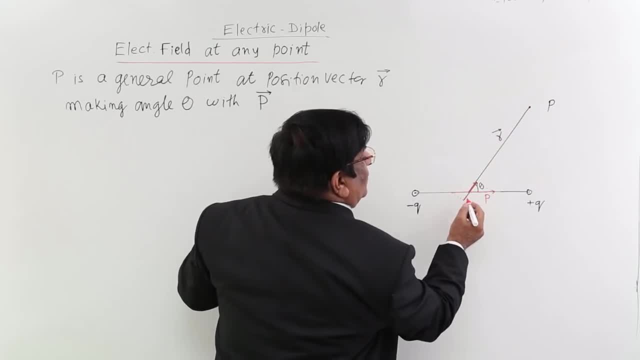 t el momento Опion is in this direction of R, so we will call it component P, which is along the direction R, or we can say parallel to R. now, where is the other component? answer: this is the other component, this, so this is basically P. this I have resolved into two components. one is this, one is this: 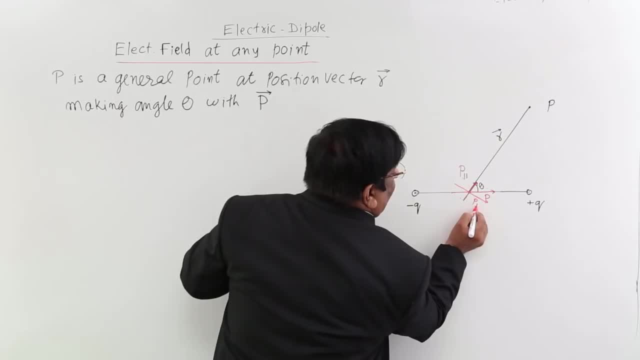 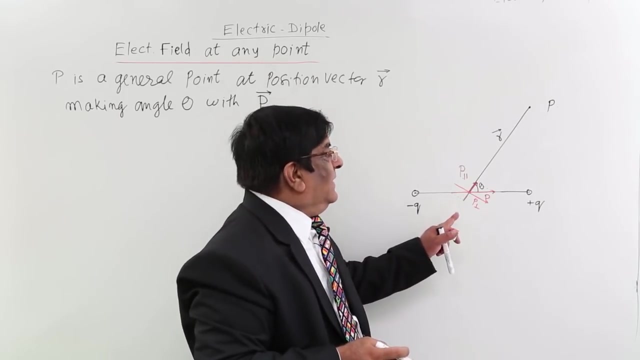 this is P parallel and this is P perpendicular- parallel to R, perpendicular to R. so this P is no divided into these two. what do I want to do? what is our line of action? in place of finding electric field due to this original P, I will find out electric field due to this. 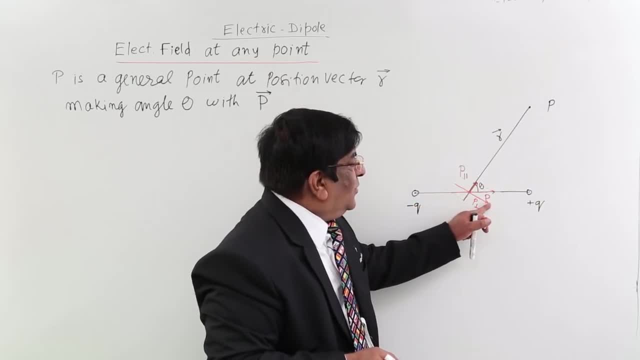 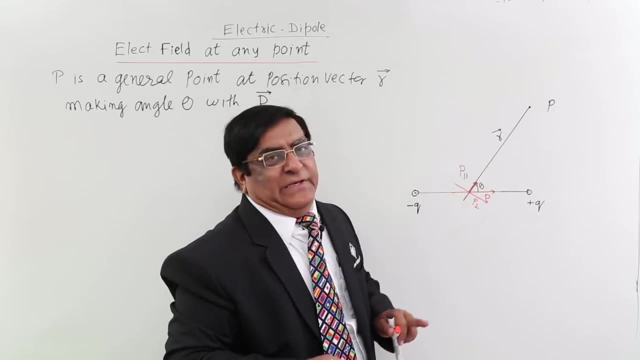 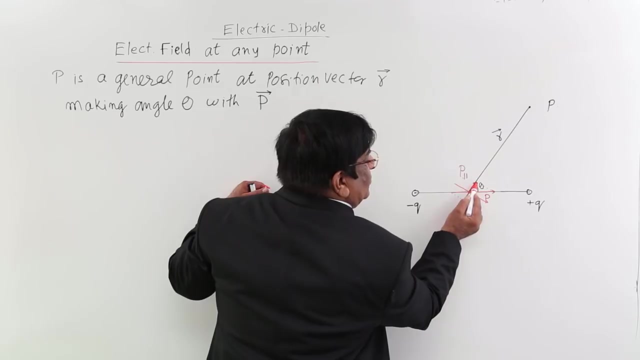 component, then I will find out electric field due to this component and then I will add up the two electric fields fields here. that will give the electric field due to complete P. So this is our line of action. So now I have to find out electric field due to P, parallel and electric field. 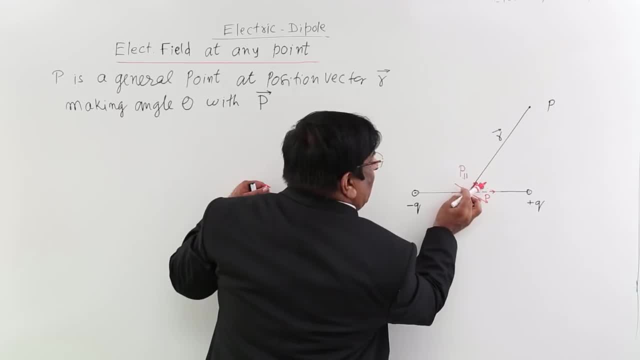 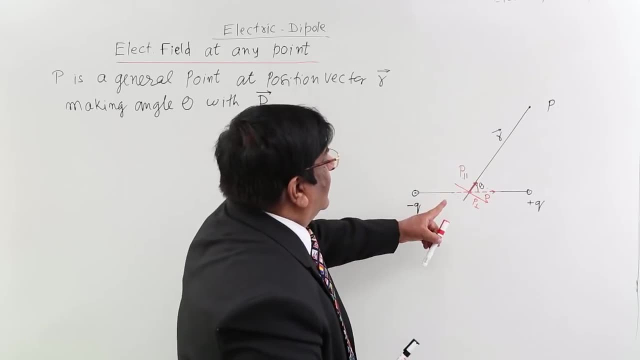 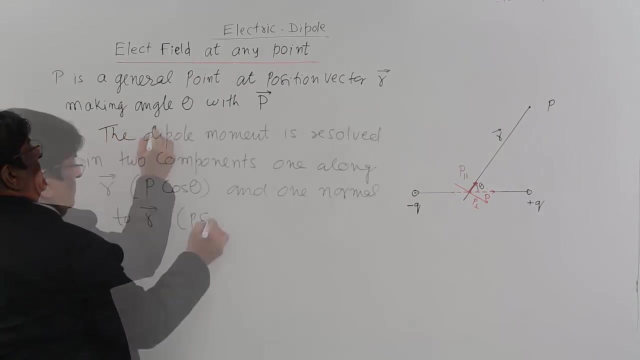 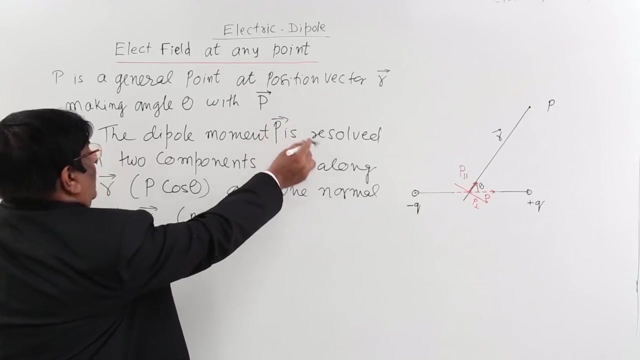 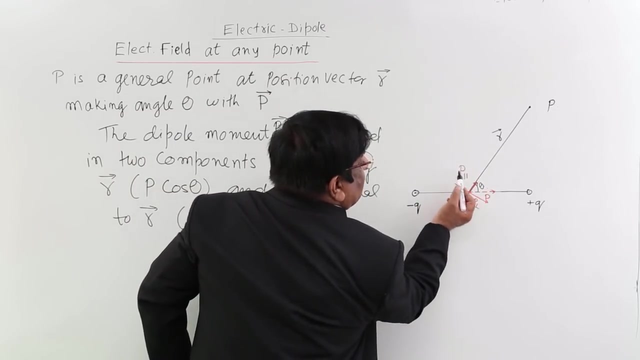 due to P, perpendicular, and that will give me the total of electric field due to this P. So we will start it this way and whatever we have done first, we will write it in one line. So the dipole moment P is resolved into two components: one along R. This is theta. 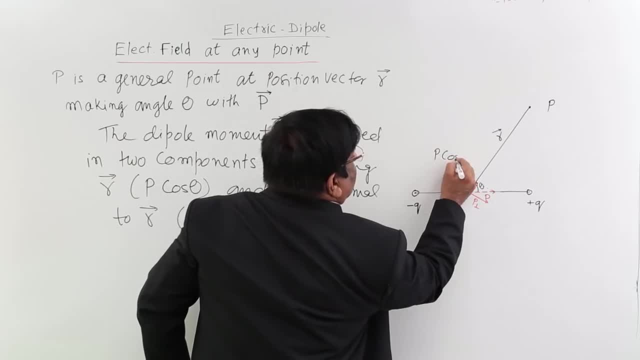 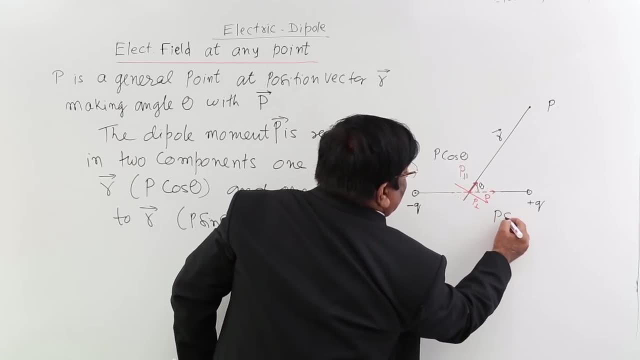 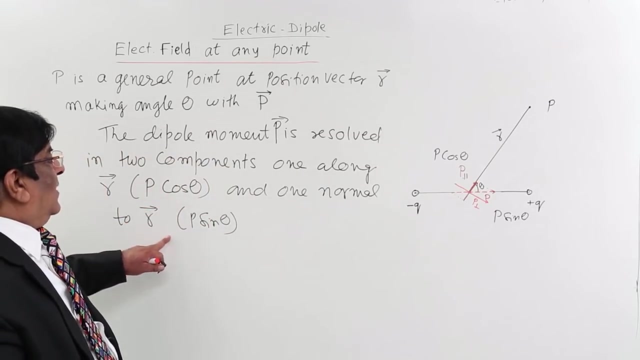 so what will be the magnitude of P parallel P cos theta? One will be normal to R this and how much this will be P sin theta. So this I have written Now along the R perpendicular to R. This is we have done so far. Now we will find out. 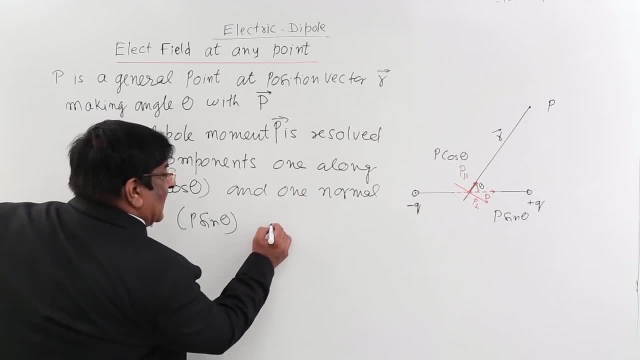 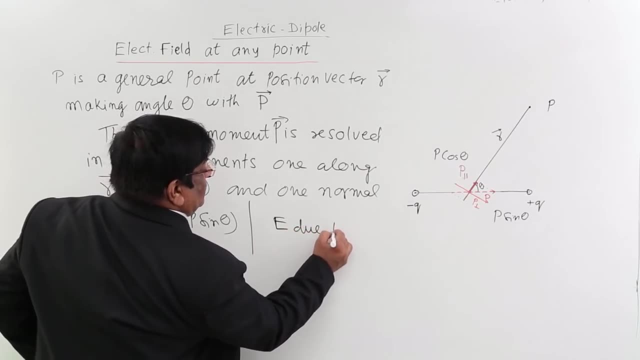 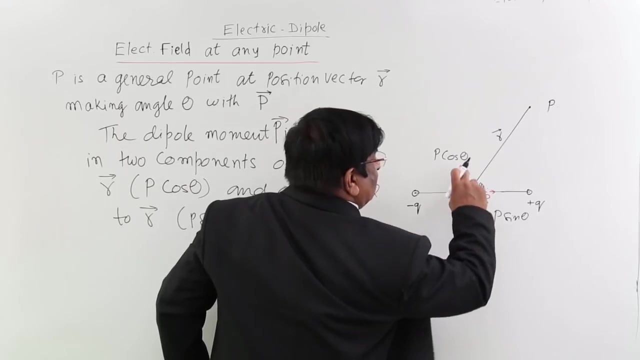 electric field due to both. So electric field due to electric field due to P parallel. Now do not see this, do not see this. see only this much: There is a dipole which has a moment, this red line, this red line. 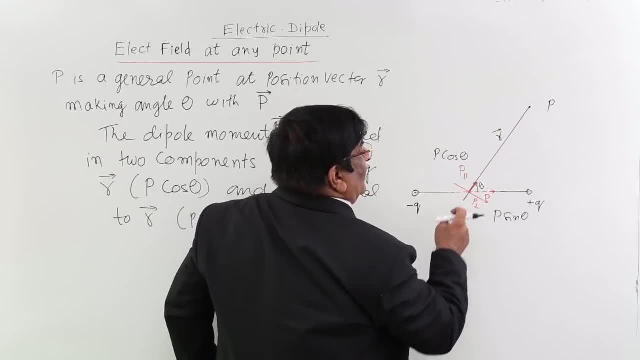 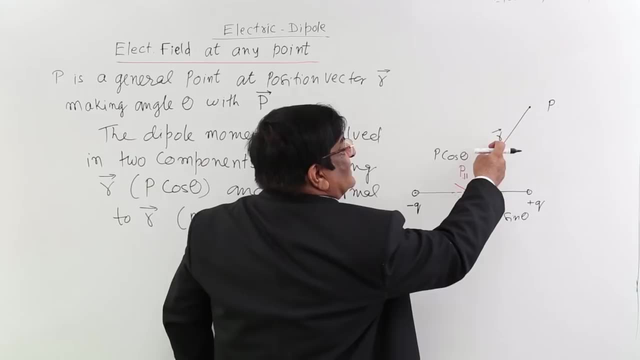 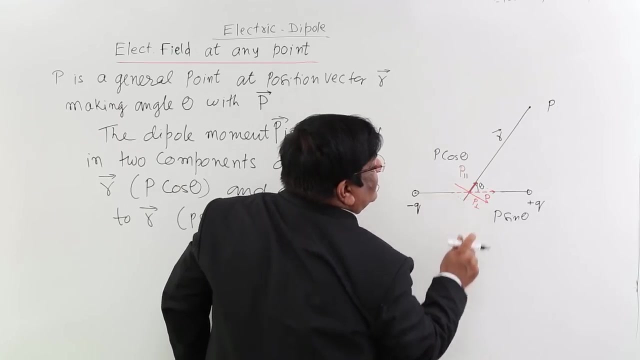 and there is a point P. You remember which situation it is. If this is P and this is the line, then we will call it x-aligned. for this P, The same line is equatorial line. for this P, Am I clear? See again, For this line, this is equatorial line. and for this red P: 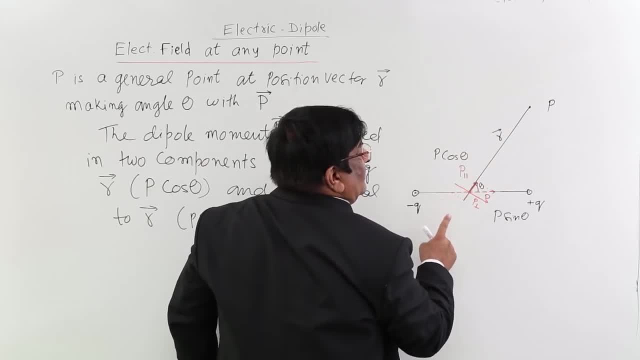 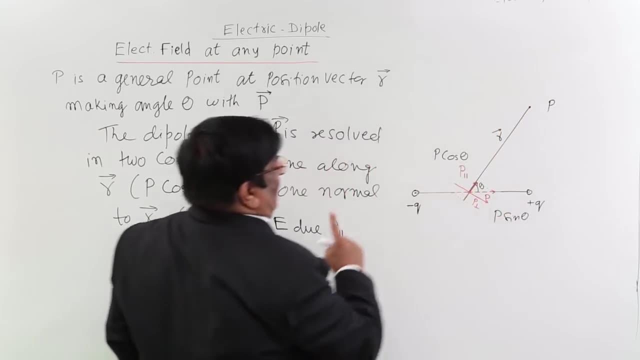 this is x-aligned. So now if I am calculating electric field due to this component, then I should use the formula for x-aligned. And what was the formula for x-aligned? That was 2P upon R, cube 1 upon 4 pi, epsilon 0. But here P does not have full value, It has a. 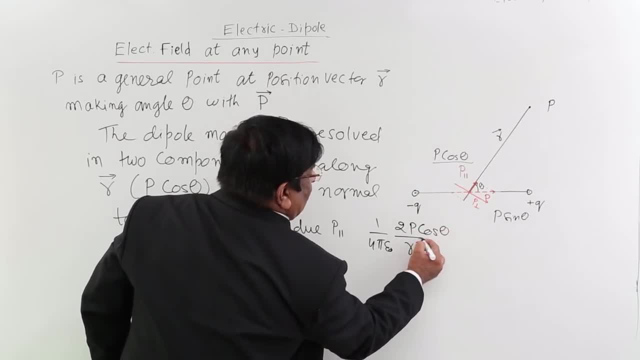 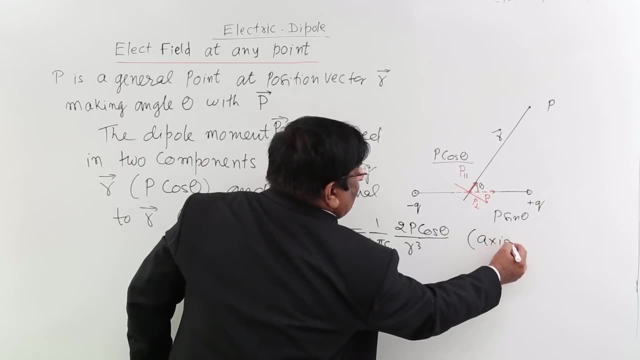 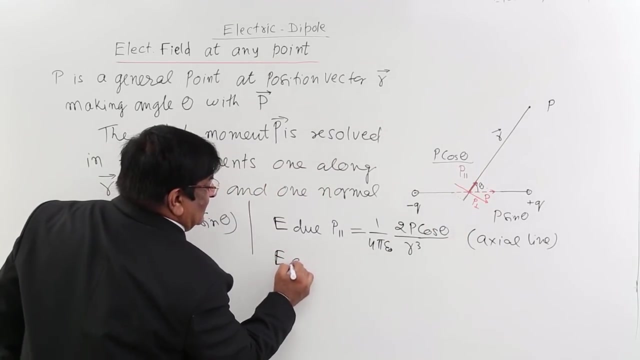 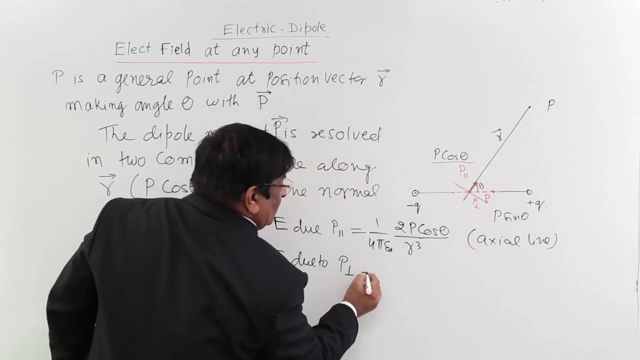 partial value. What is that? P cos theta? So this is E due to P. Why x-aligned? For this it is on the x-aligned, Then E due to P- perpendicular. For this P it is on the equatorial line. So I will use the formula 1 upon 4 pi, epsilon 0, component. 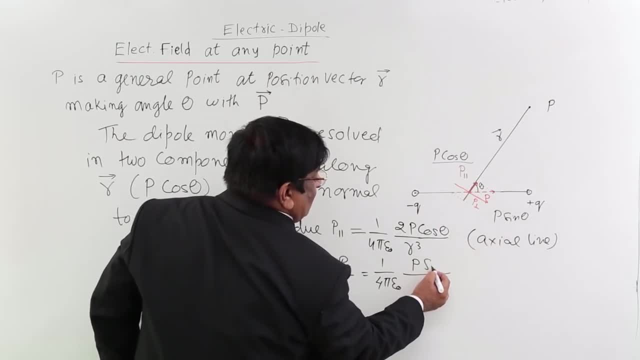 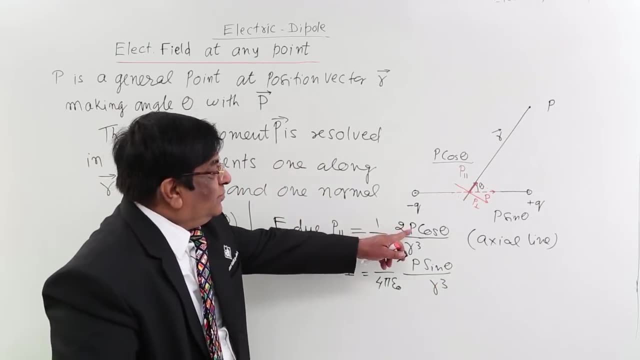 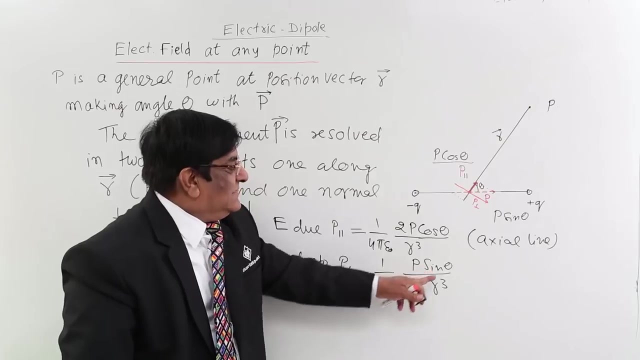 of the P, Which component? P sin theta, P sin theta divided by R cube. This you have done earlier. This is 2P, This is 1P, And here P value is P cos theta And for this equatorial it is P sin theta. Now, this, our electric field. What is the direction? 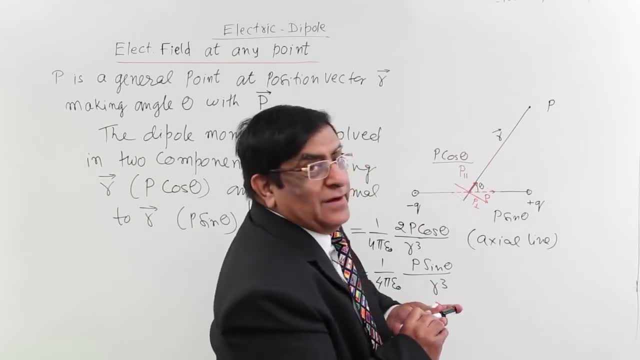 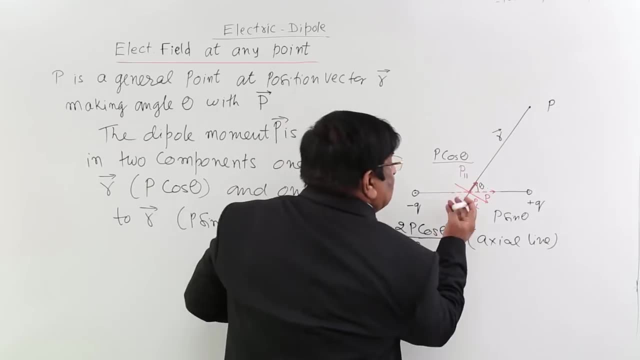 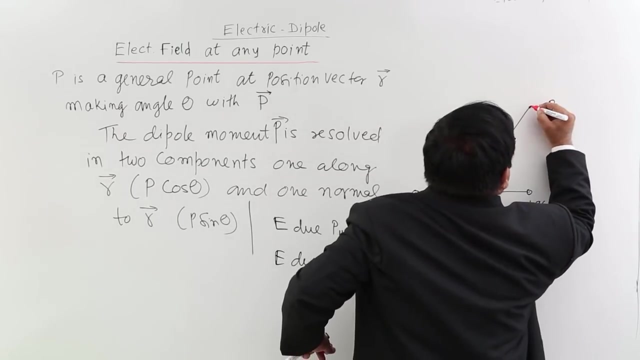 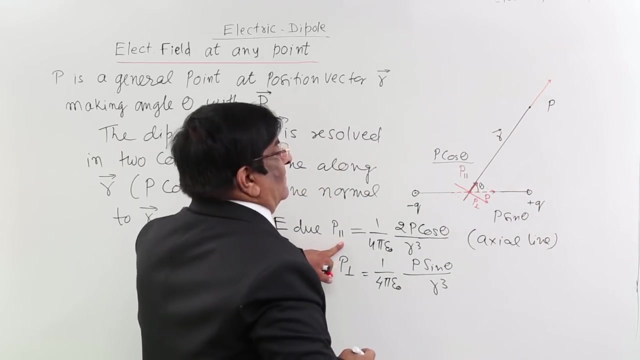 of electric field here. For that, I remind you, For x-aligned, what is the direction? we remember It is along P. This is the P for x-aligned line effect. So this is the direction of this electric field due to P parallel. I will. 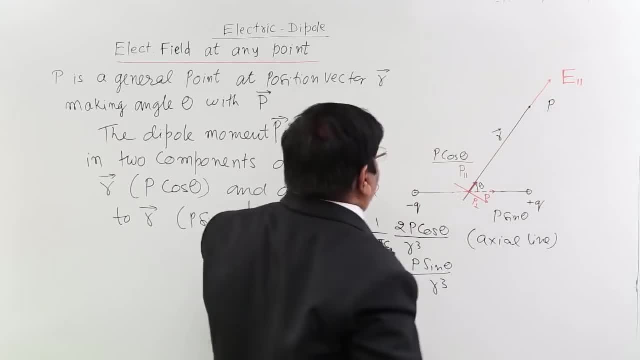 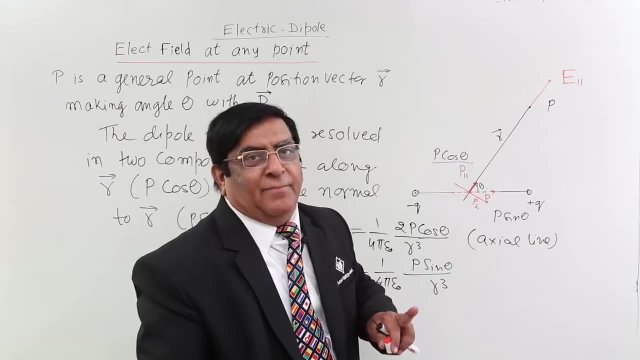 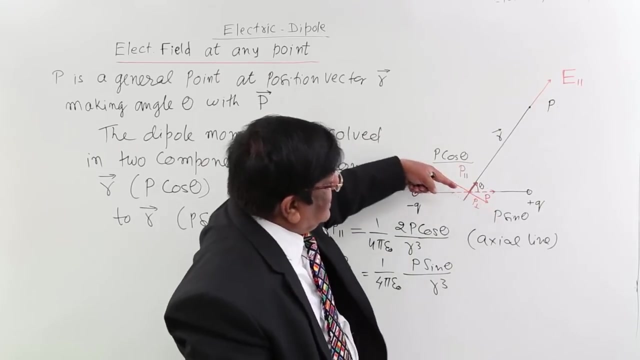 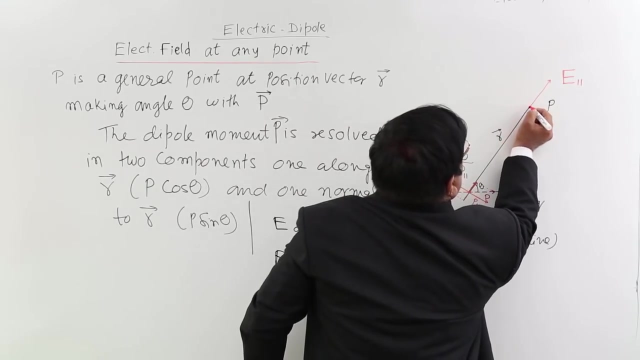 write it: E parallel. Now this P perpendicular. this is on the equatorial line and what we remember for equatorial line direction of E is opposite to P. If P is in this direction, then electric field will be in this direction, opposite to this. So here it is opposite. 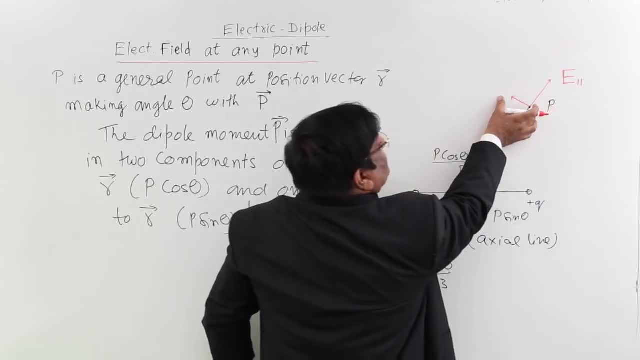 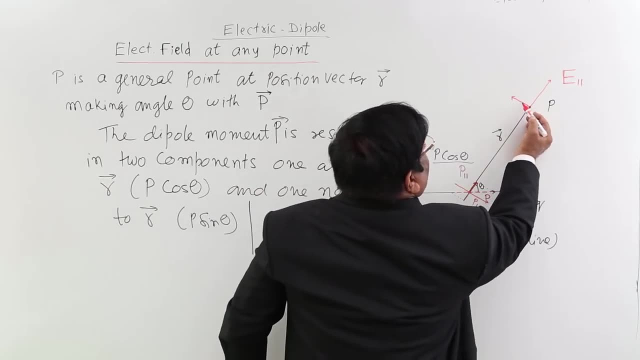 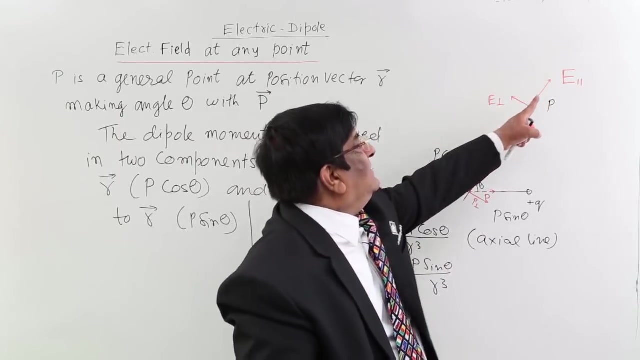 to this and it is a bit small. Why small? Because it is 1P. The rest depend upon theta Anyway. so this is E on equatorial line. So we have done this. We have one E this, one E this. this has got magnitude. this much, this has got magnitude. 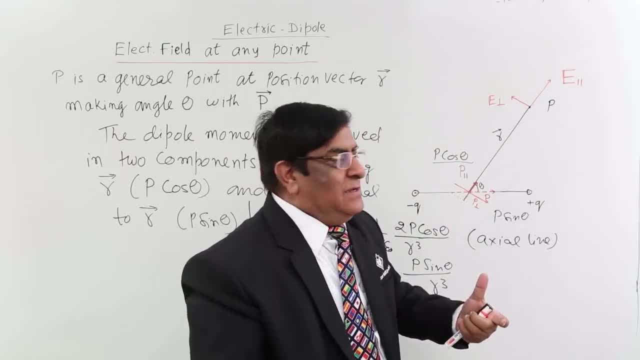 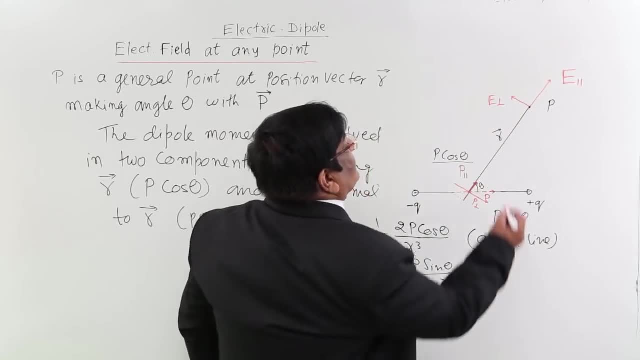 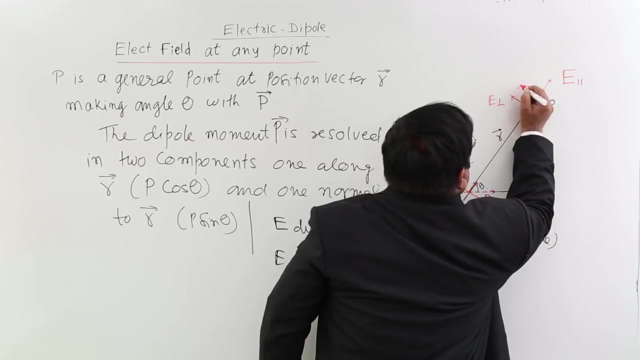 this much and due to our earlier training, earlier lesson- we could find these magnitudes and these directions at point P. If these are the two electric fields at point P, we can always find out a resultant. How do we find out a resultant? We complete the parallelogram. 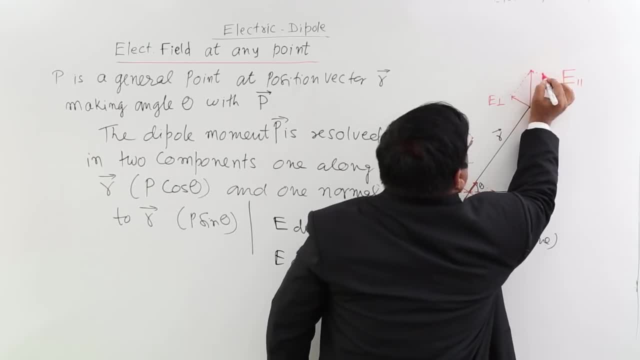 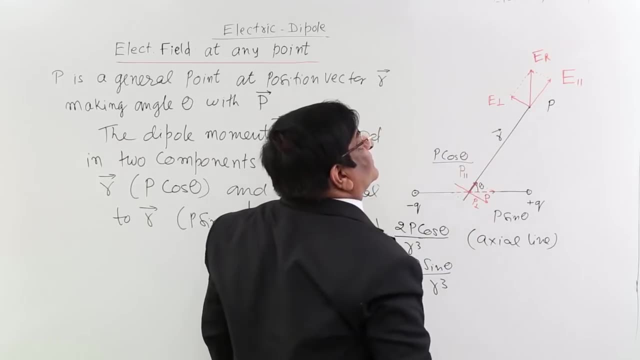 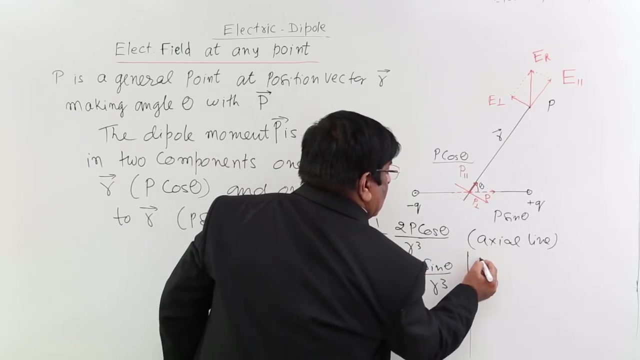 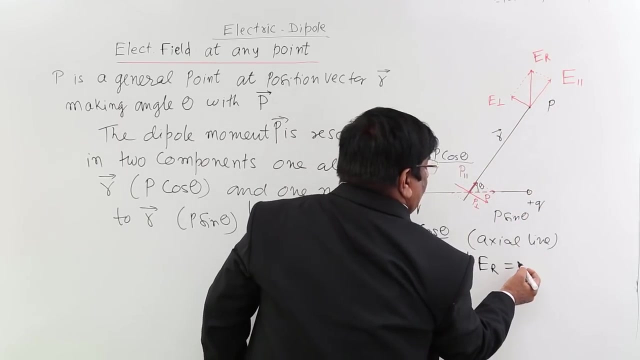 and we can look at the resultant E. These are E and P. Now what is the E resultant? We can do it like this: This E is a point P, This is the E resultant, this is the E resultant. So this gives us E resultant, E resultant at: 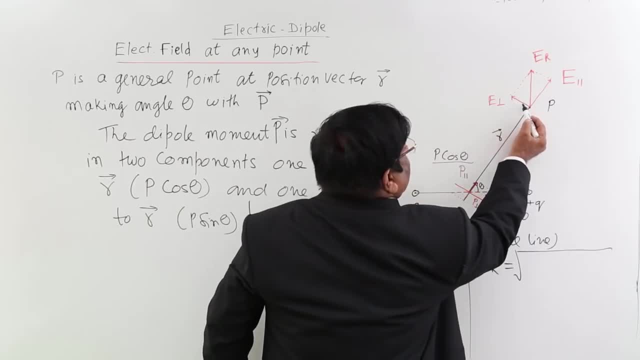 the point P. Now how much is this E resultant? So this we can write here: E resultant is equal to. these two are making right angle to each other, So this will be very simply square root of square of this plus square of this. So E resultant is equal to. P is the 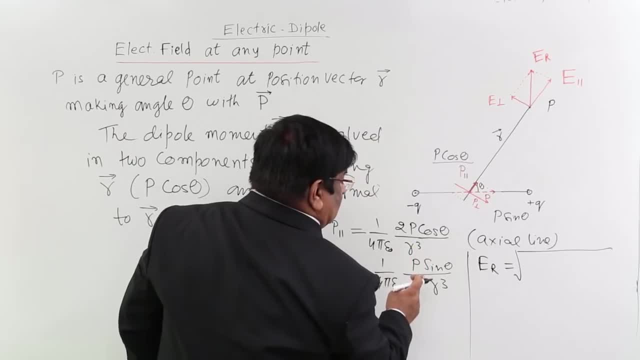 earlier angle. Now, how much is this E resultant P? So this is, P is equal to right angle to. So this is square of this plus square of this. I will go straight writing the square. This square will be this whole square. E resultant is equal to square root of square of the first. 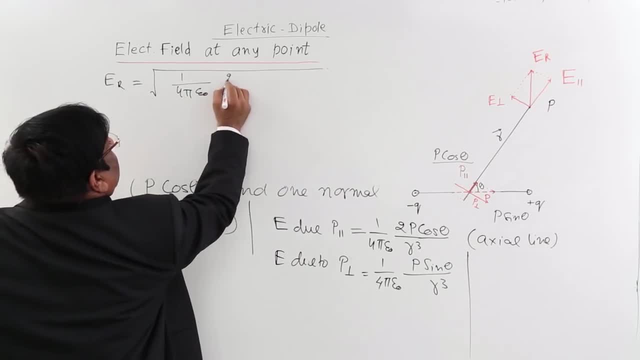 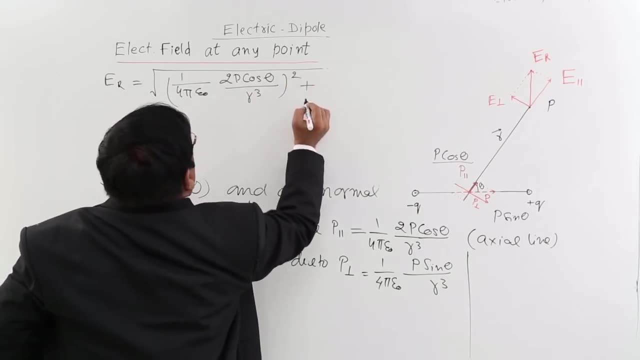 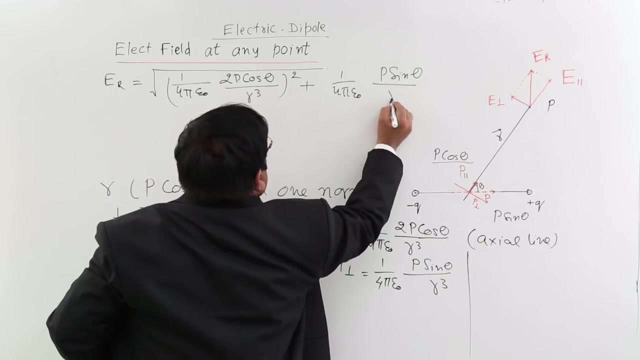 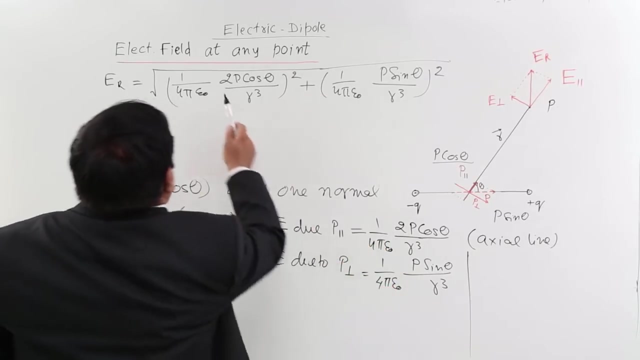 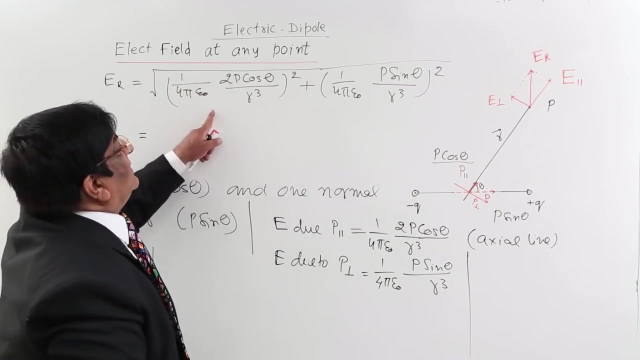 term: 1 upon 4 pi epsilon 0, 2 p cos theta upon r cube square of this, plus 1 upon 4 pi epsilon 0 p sin theta upon r cube square of this second term, This square, this square, square, root of the two, Now, this and this are common. Their square is common, comes out of the square. 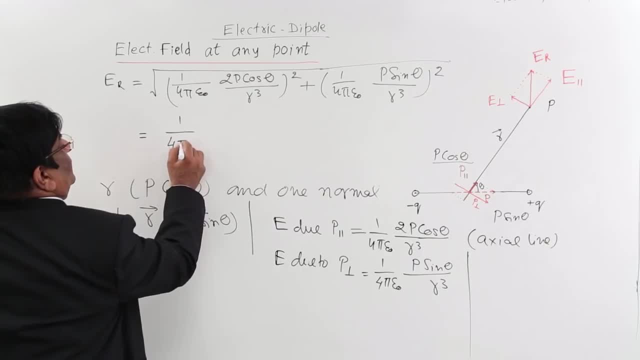 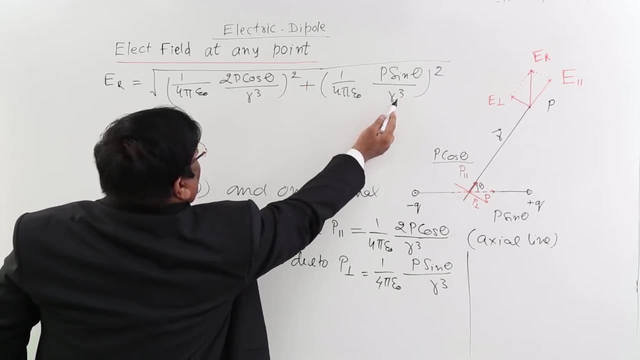 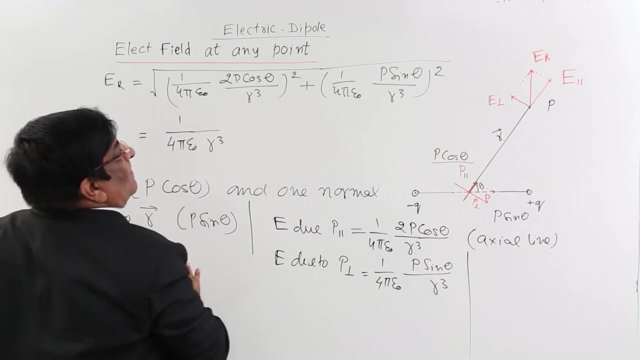 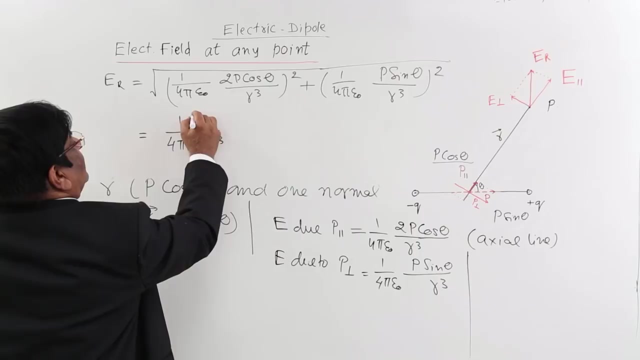 root and what we get here is 1 upon 4 pi, epsilon 0.. Your mathematics will confirm it: r cube square. R cube square is common taken out of this square root. so we get here: R cube. they come out Again P square. P square taken, common, coming out this will be P. 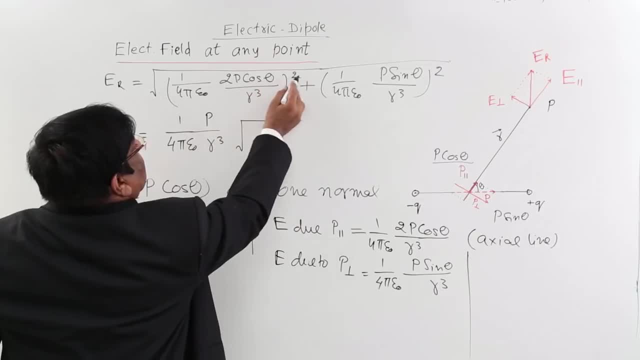 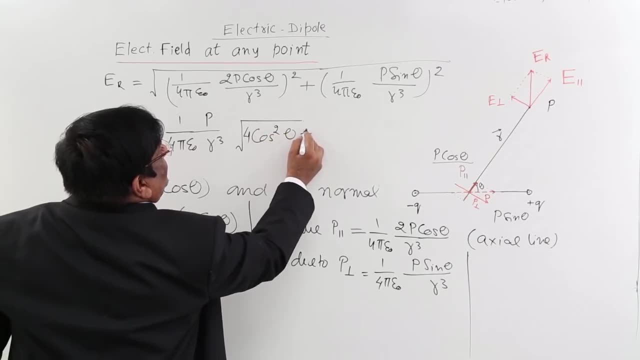 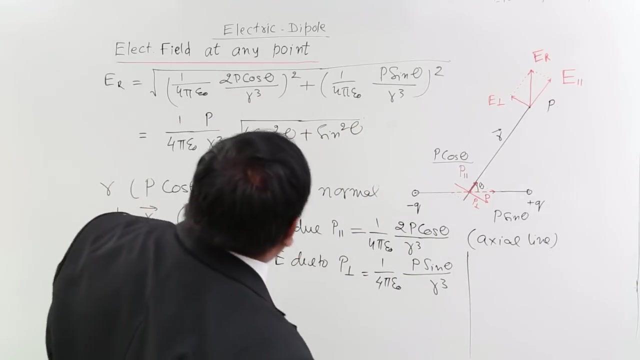 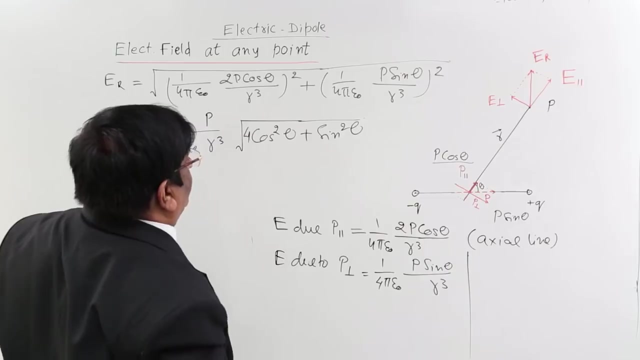 Now what remains inside is cos theta square 2 square, so 4, cos square theta plus sin square theta. and now you all know that sin square theta plus cos square theta, that is equal to 1.. So this we can write as 1 upon 2.. 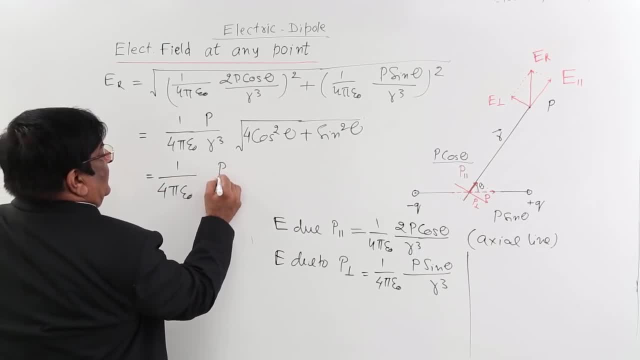 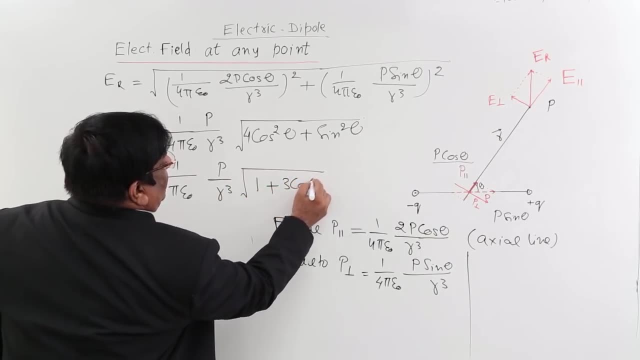 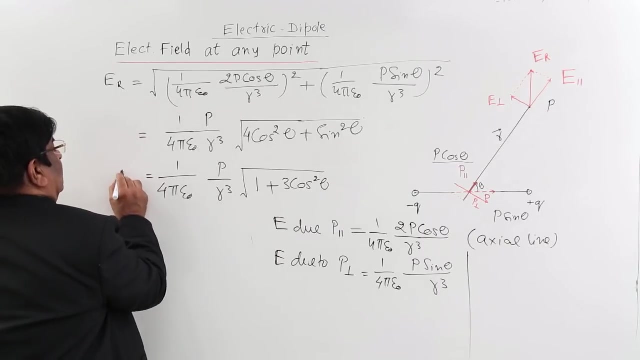 Okay, Okay, Okay. So this is 4 pi. epsilon naught P upon R cube, and this will be 1 plus 3 cos square theta, 1 cos square theta and 1 sin square theta makes 1, and this is our E resultant. 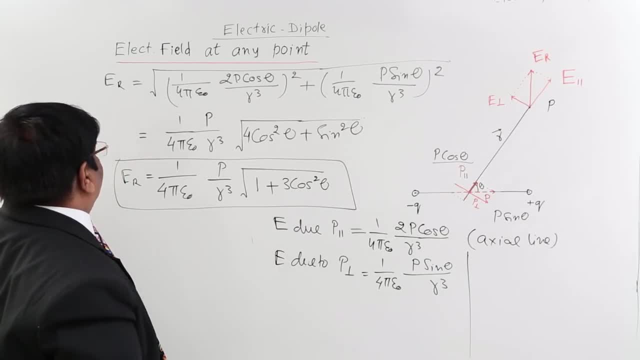 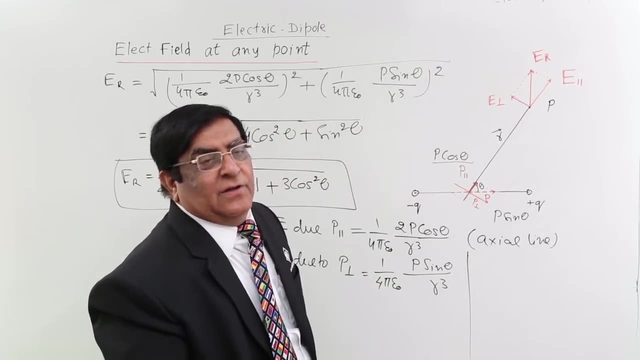 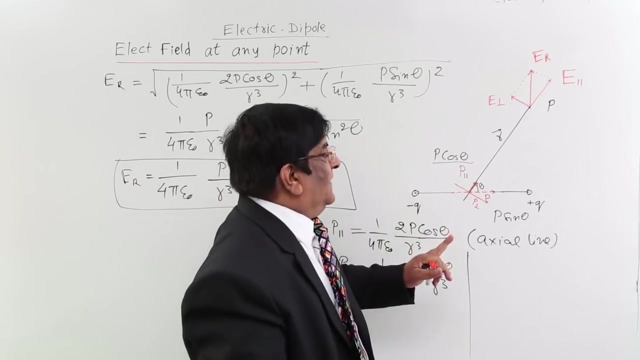 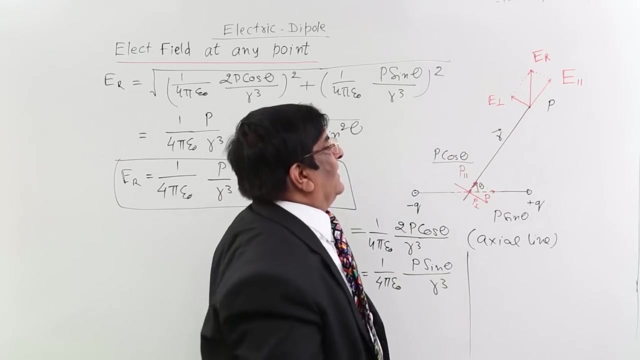 This is magnitude of E resultant. This is answer, then what should be its direction? For the direction, we have to first fix up a reference line. Here we fix up, we have two reference line, one is P, one is R. So here R is easier to find out as to make as a reference line. so this is our reference. 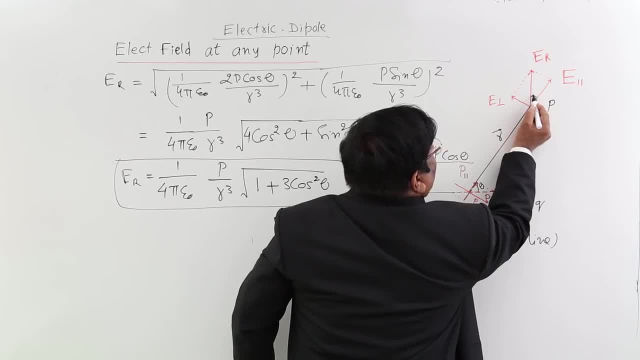 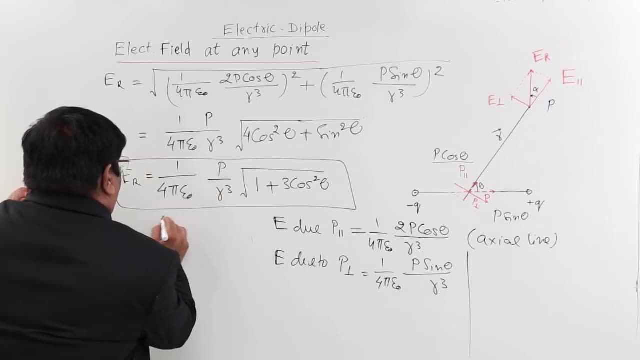 line R and this resultant makes certain angle with R. let us say this angle is alpha. So this resultant makes any angle alpha, angle alpha with r. this resultant makes angle alpha with position vector r. and now we have to find out value of alpha. so for value of alpha we write. we take that triangle in this: 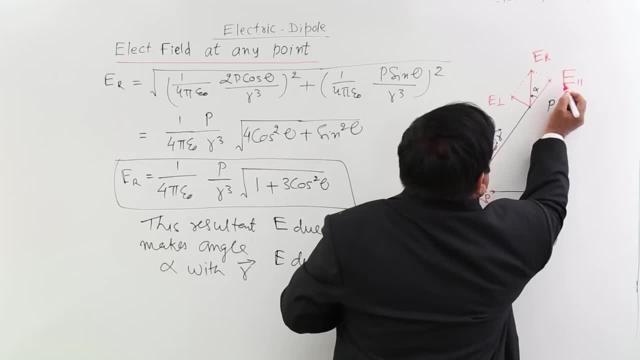 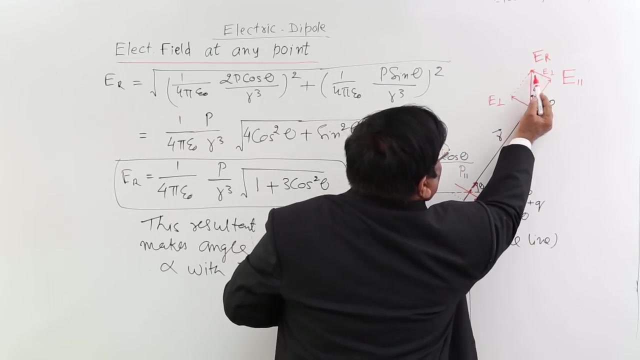 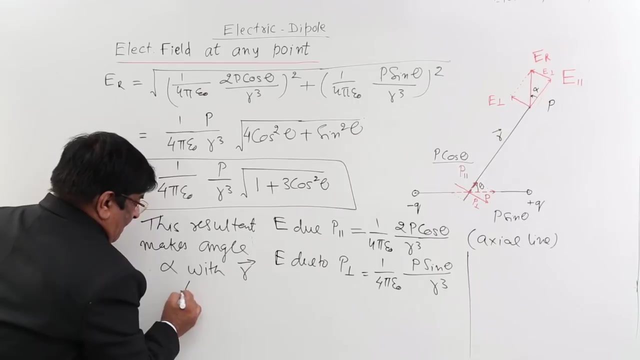 triangle c. this represents e parallel and this is e normal. if i draw a line here, this is equal to this. so this is also e normal. this is e resultant of course. so tangent of alpha is perpendicular upon base. so here i have tangent alpha. tangent alpha is equal. 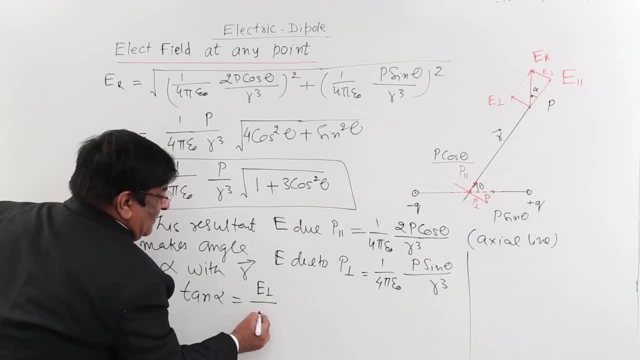 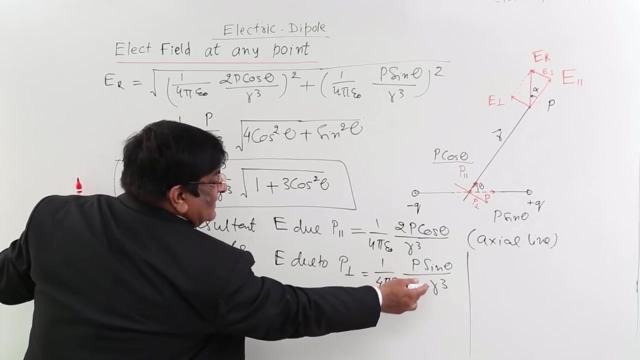 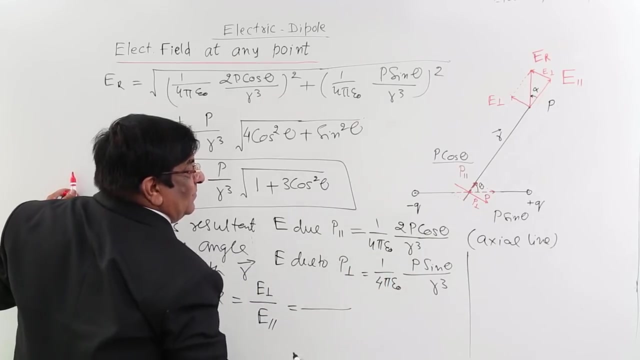 to e perpendicular upon base. Now, how much is e perpendicular? e due to p perpendicular, is this so? this is 1 upon 4 pi epsilon, not p sine theta upon r cube and e parallel will be this: you can cancel out here everything, and what will be remaining? it will be remain here e, parallel sine theta. 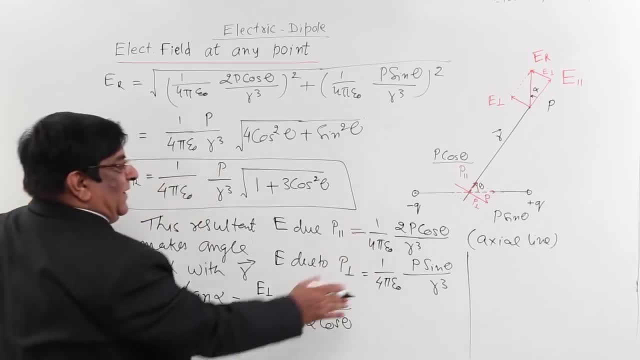 and here will be intermedi images. So 1 upon 4 pi epsilon, 1, omega of p, sine theta upon r square. and what? how can this happen? now, here it will be 2 cos theta, you can make it e parallel to rest. everything will be cancelled. 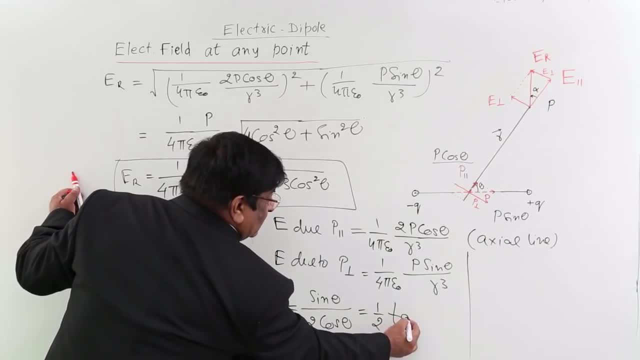 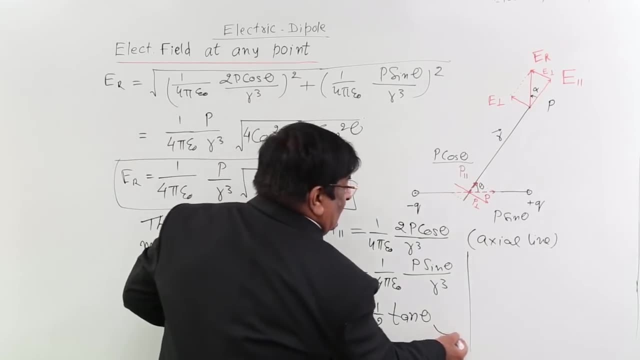 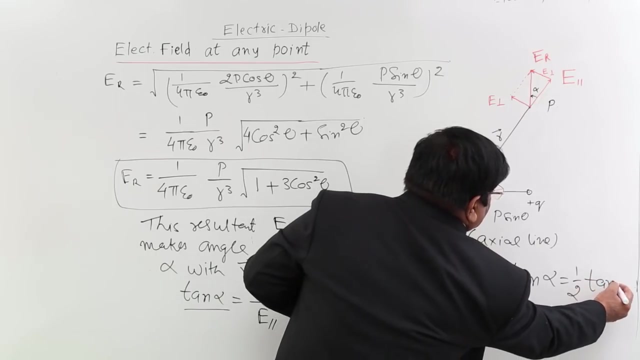 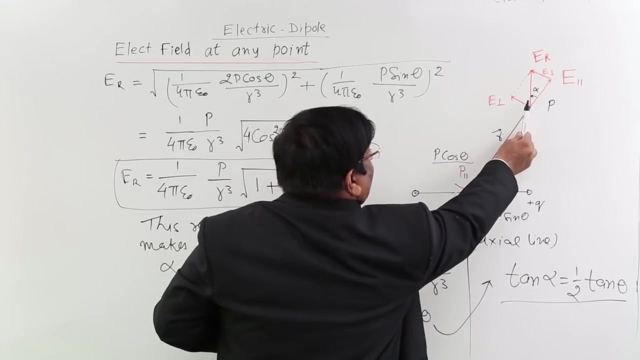 so this is equal to half tan theta. so tan alpha is equal to half tan theta. lets jump here. tan alpha is equal to half tan theta. theta is the angle of position vector. with p, the resultant will be in such a direction that alpha with r will maintain this relation. 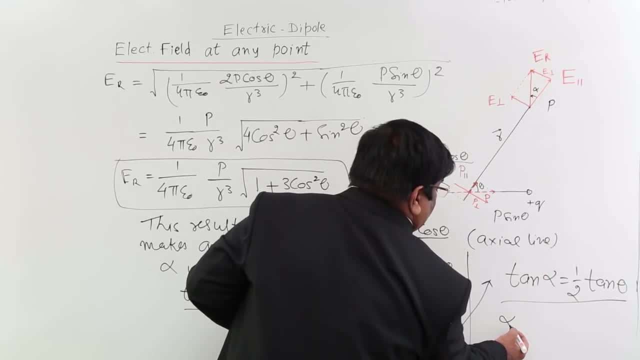 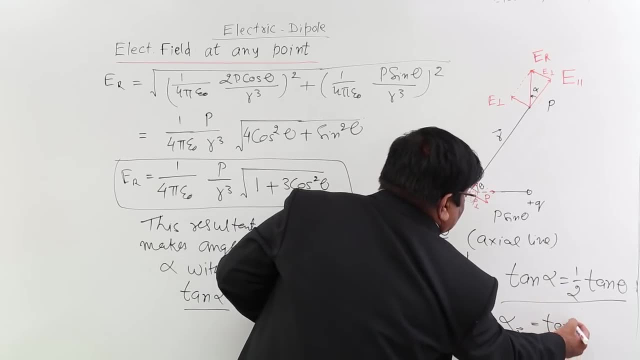 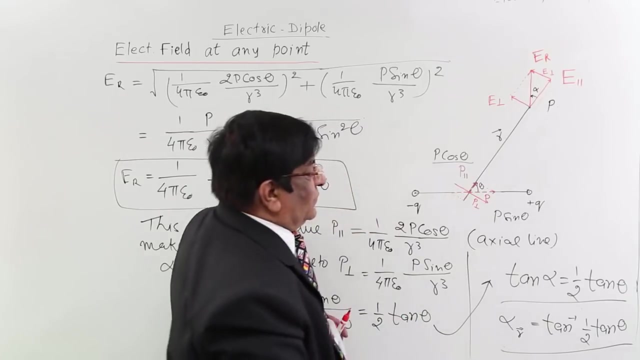 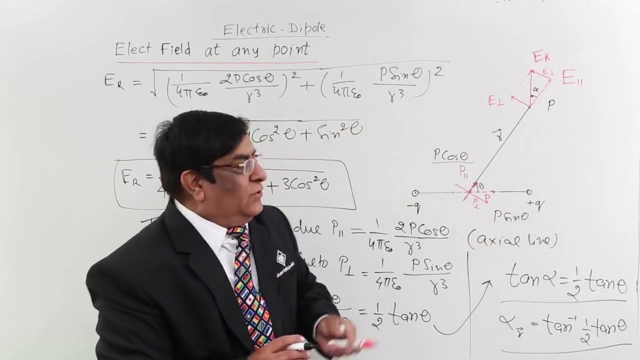 half of tan theta. so we can always find out alpha with reference to r vector. this is equal to tan inverse of tan alpha, or half tan theta inverse, half tan theta. So this is how we can find out direction of the resultant with respect to position vector. So now you get for any general point. this is magnitude. 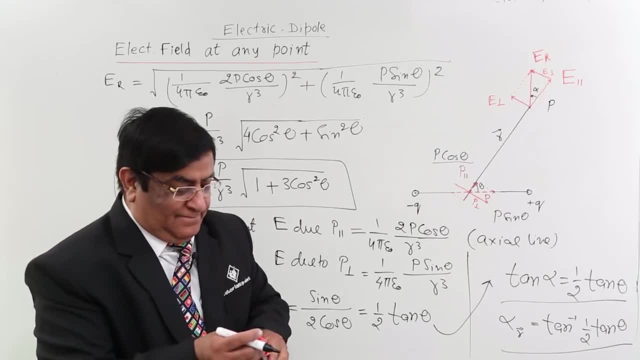 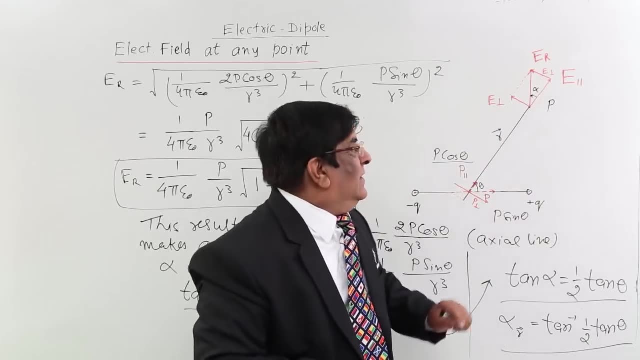 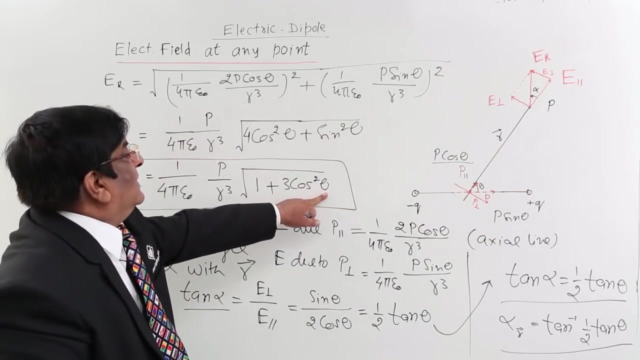 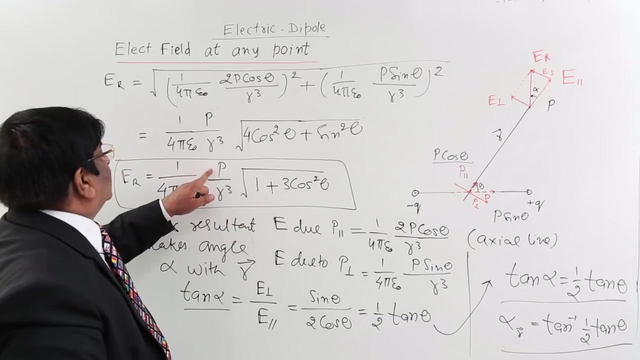 this is direction. Want to test it. Yes, If it is an axial position- suppose P is here- this is an axial position. What is value of theta? The theta will be 0 and you put 0 here. If you put 0 here, cos 0 is 1, this will be 3, 3 plus 1 is 4, 4, square root is 2 and this. 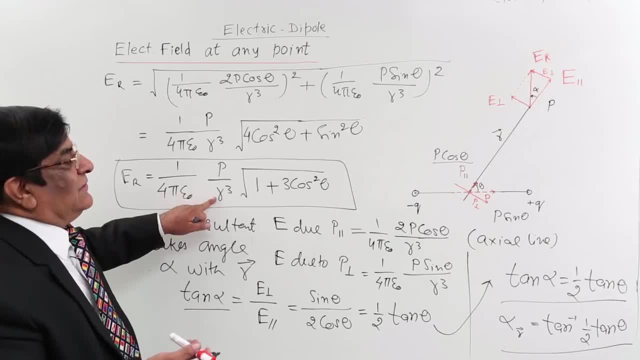 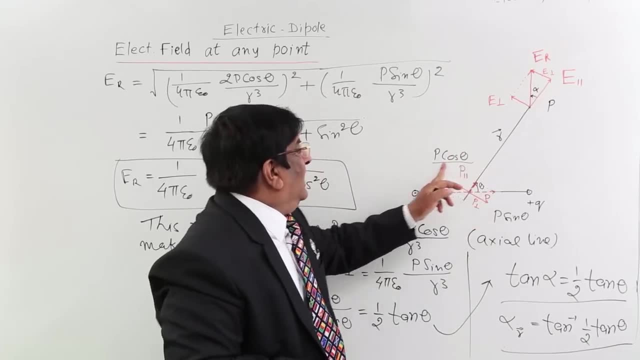 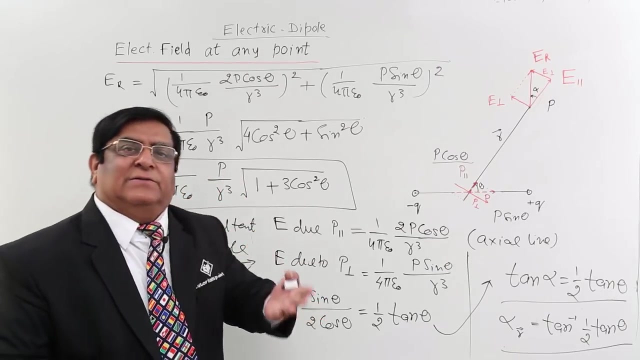 will be 2 P upon R Q, and we know that that is the electric field at the axial line. If you want it on equatorial line, theta will be 90, this will become 0, theta will become root. 1 will be 1, this will be 1 P upon R Q. we have learnt that is on the equatorial. 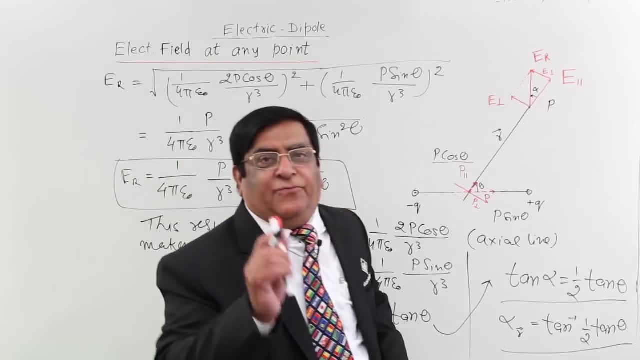 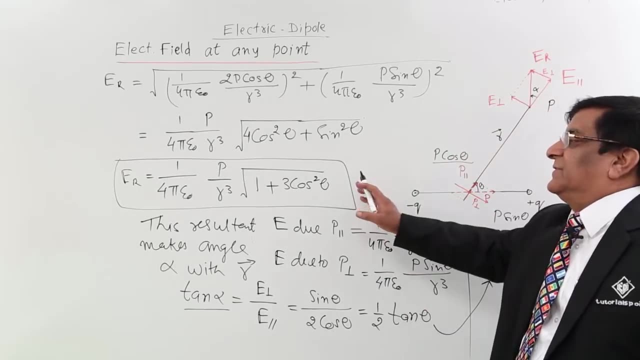 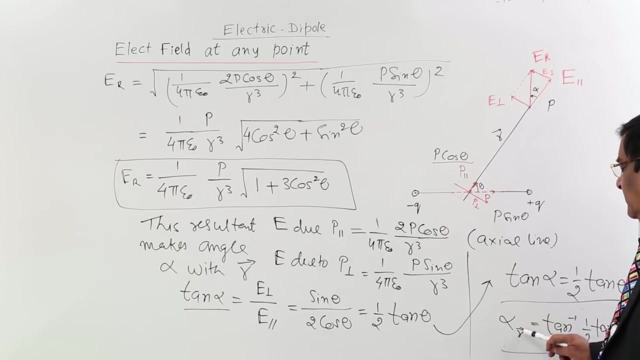 line. So this is a general formula which will fit on axial line, on equatorial line, on any general angle making theta. So this is known as general formula for electric field due to a dipole and accordingly we can find out alpha for that resultant electric field.